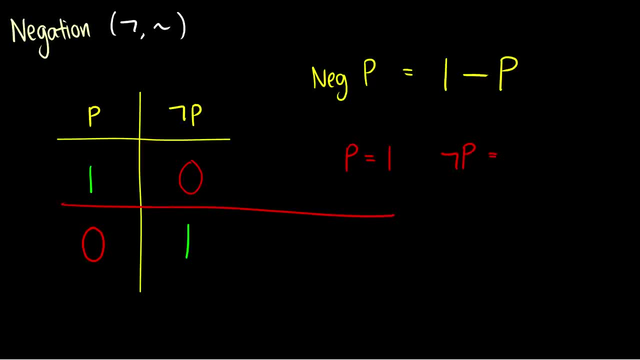 row here then not. p is equal to 1 minus p, which is just equal to 0. So that's a nice mathematical way we can find the value of the negation. Let's take a look at connectives that involve more than one statement, So for example, conjunction. 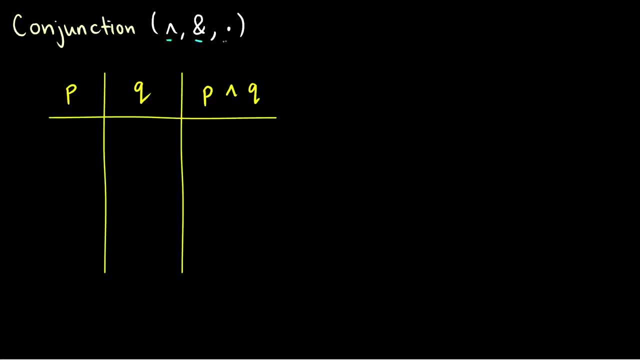 And you will see either the caret, the and symbol or the dot for conjunction. I will always use the caret because it's typically used in most discrete math texts. So here, conjunction: it takes two statements and combines them. So how do we build a truth table? 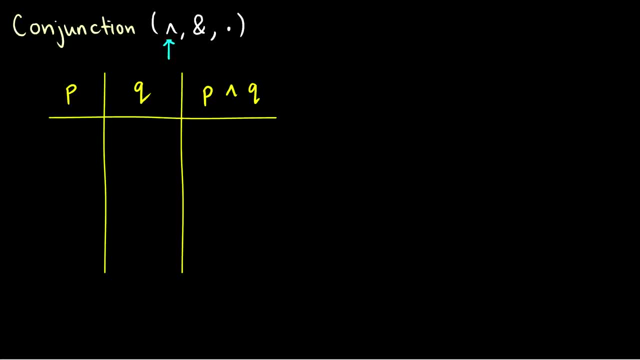 for two statements. Well, Q can either be true or false, And P can be true or false. So all possible combinations. well, Q can be true-false, true-false, And then P. well, there's two situations where P will be true and two situations where 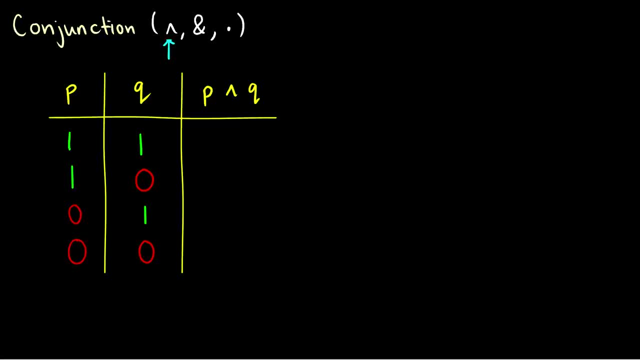 P will be false, And now we can see that we have all possible combinations of P's and Q's. So if we have two statements, we need four rows, because each one can be true or false, which means that there's two possibilities for Q. 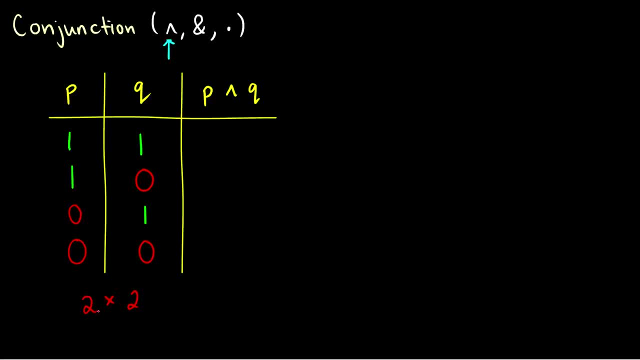 and two possibilities for P, which means we need four rows. If we had another statement, R, then we'd need another doubling, because R can be true or false and we need eight total rows. So the number of rows is equal to 2 raised. 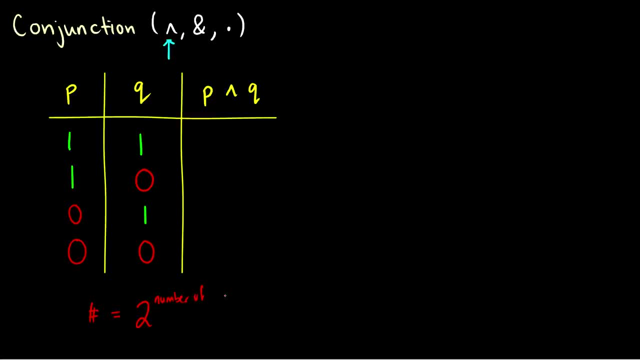 to the number of statements. So that's just building a truth table. Now, what does P and Q do to the truth value? Well, P and Q is true only if P is true and Q is true. So it's only true in the first scenario, where both P and Q are true. 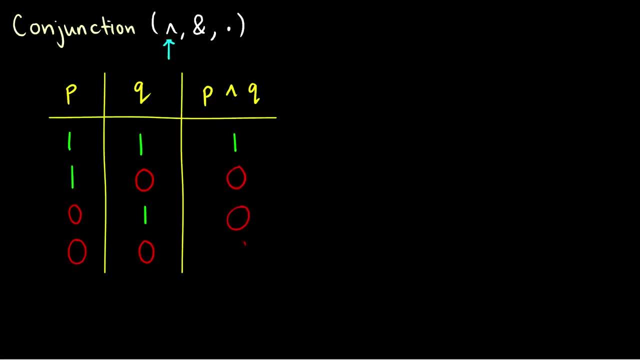 In every other scenario it is false. So what's the mathematical way of looking at this? Well, we say that the value of P and Q is just equal to the minimum of P and Q. So, for instance, the minimum of P and Q in the first row is: 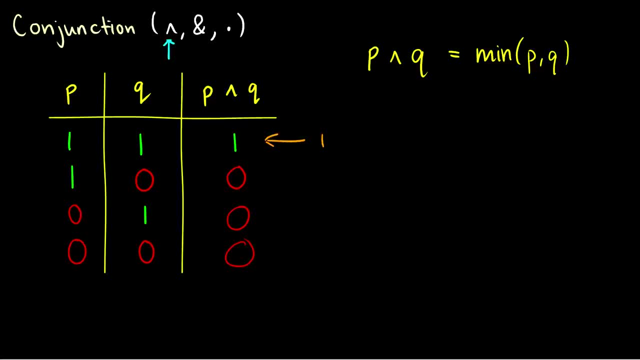 1, because the lowest value is 1. In the second row, the minimum of P and Q is 0 because Q is the lowest value. In the third row, P is the lowest value at 0, and in the fourth row, both p and q are zero. So that's conjunction. and of course conjunction is, and Let's take a: 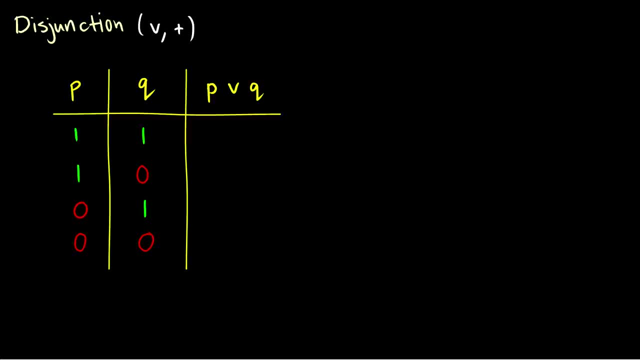 look now at disjunction and disjunction. you'll either see the v or you'll see a plus sign, the plus sign more in abstract Boolean algebras. But what does p or q do? Well, p or q is true if at least one of p? q are true, which means in the first row is true, because both are true. 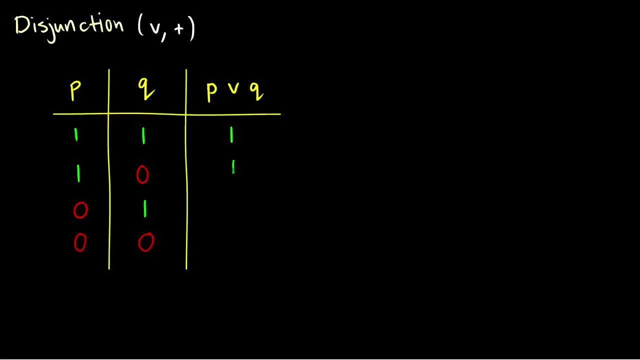 in the second row, it's true because p is true. in the third row, it's true because q is true, but in the fourth row neither p nor q are true. therefore p or q is false. So again, mathematically we can think of this as p or q. just takes the. 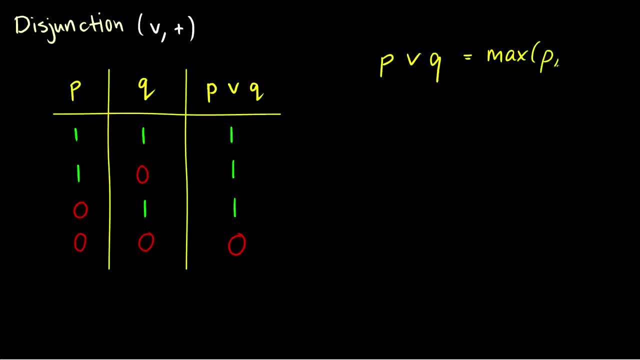 maximum of p and q. So in the first row both are ones. one is the highest value, so it's true. in the second row, p is a one. that's the highest value, therefore it outputs a one. in the third row, q is a one, which is the highest value, which means it outputs a one. but in the fourth row, 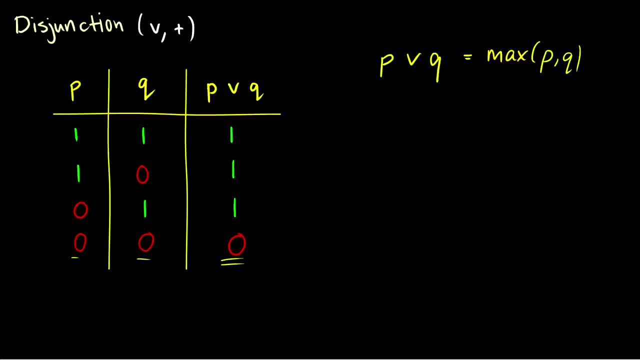 the highest value is zero, so we output a zero. that is disjunction. Now what about the conditional and the conditional? we usually see the arrow and occasionally we see the superset symbol, but this is more for philosophical logic and not seen too much in any math texts. So this is an 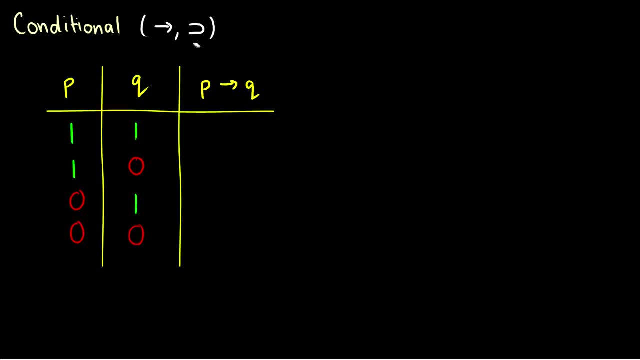 interesting one. this is the truth condition, for if p, then q, and it is only false. if p is true and q is false, the rest of the times it will be true. and this is kind of hard to wrap our brains around, and I'll emphasize this more in an upcoming video on just conditionals on their own. But for now let's say that I 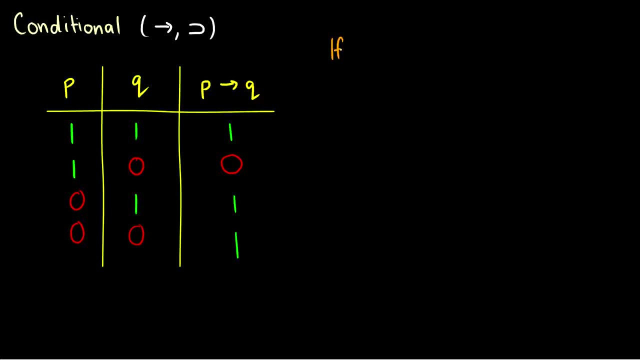 tell you, if it's sunny, I will wear sunscreen. So let's say: I tell you this: when am I lying to you? I am lying to you if it is sunny out, which would be, P is true, and I'm not wearing sunscreen. This is like my promise to you. I'm 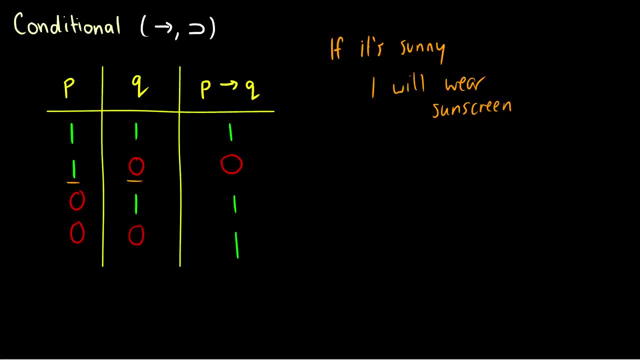 saying: look, if it's sunny out, I promise I will wear sunscreen. And if it is sunny and I'm not wearing sunscreen, I lie to you. Therefore, the conditional is false. But if it's not sunny outside, well, I'm not lying to you, am I? It doesn't matter if I'm wearing sunscreen or not. 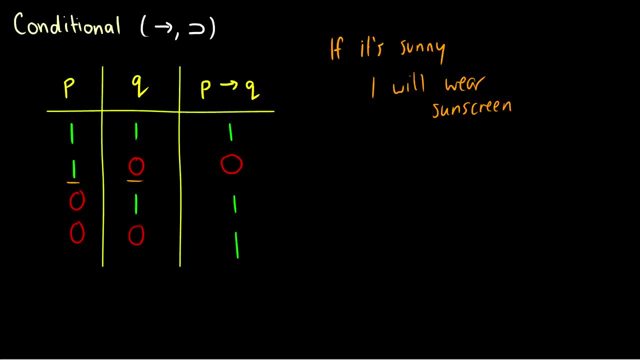 It's not sunny outside. Therefore I'm not violating any truth conditions. Therefore it is true in the bottom two cases, And this is a very difficult thing to wrap our heads around because we think, well, if it didn't happen, then we can't say it's true or false. But think of the 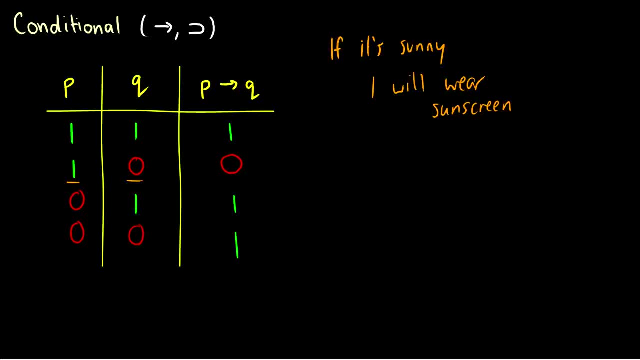 conditional in terms of when am I lying to you? I'm only lying to you in this one situation. So we say that, mathematically anyway, P arrow Q is 1 if the value of P is less than or equal to Q. So in the second scenario here, 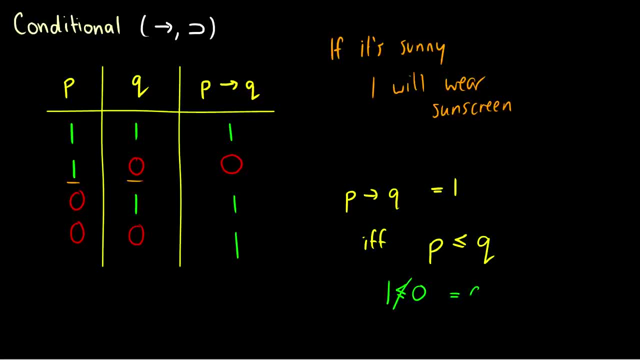 1 is not less than or equal to 0. Therefore we get a 0.. But everywhere else P is less than or equal to Q, So we output a 1.. And that's a mathematical way of looking at things. If 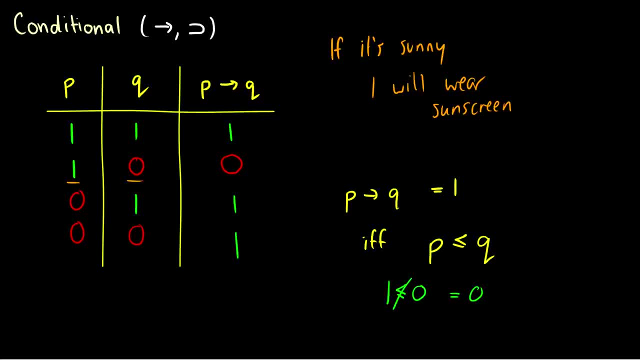 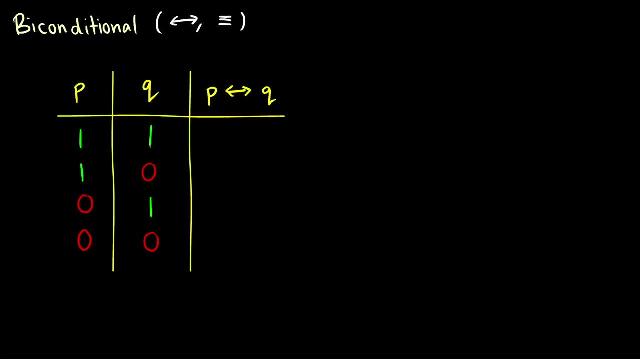 the explanation. reasoning is just a little bit too confusing or maybe you don't accept it. you can use the terms of these mathematics here. So those are the four main connectives and their truth tables, But there's two more connectives that we can define. in terms of the other connectives, 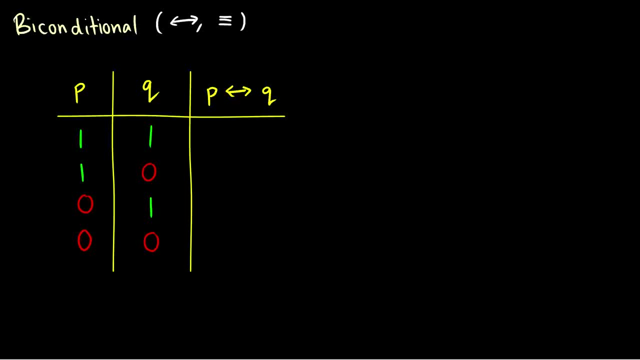 But let's just treat them as if they're their own connective. for now, The first one is the biconditional, And this is usually if and only if. So this is written if, with two Fs, or just if and only if, And typically we'll use the double arrow here. 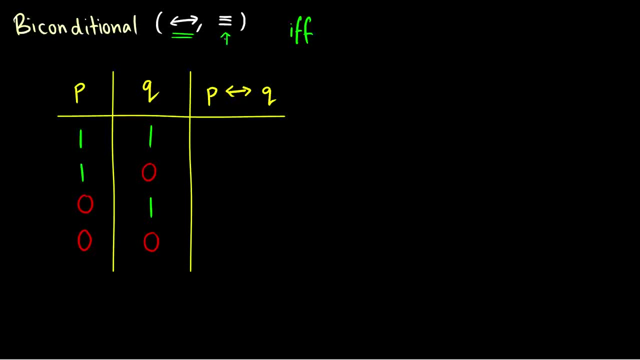 However, some texts use the equivalency symbol. This is like kind of weird to use. I would never use this myself, but I've seen it before So I'll write it here, just in case you encounter it as well. And the way P and Q works, or P if, and only if, Q works, is: if P is equal to Q, then we have 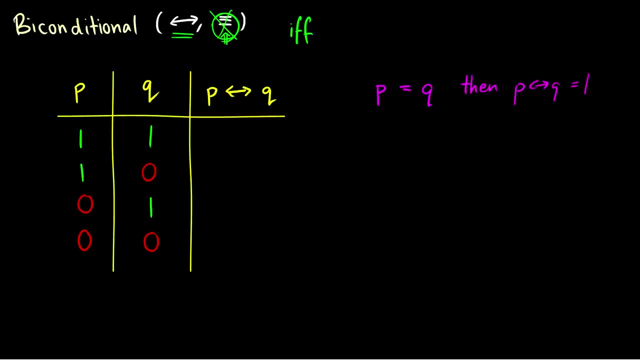 that P arrow Q is equal to 0. So if P is equal to Q, then we have that P arrow Q is equal to 0. So if P is equal to 1. So if they're the same value, it outputs a 1.. So when P and Q are both true, the biconditional is true. And when P and Q are both false, the biconditional is true. If the values are separate or different from each other, then it's false. So in the second row, P is 1 and Q is 0. Therefore it outputs a 0. If P is 0 and Q is 1, it outputs a 0, because the values aren't the same. 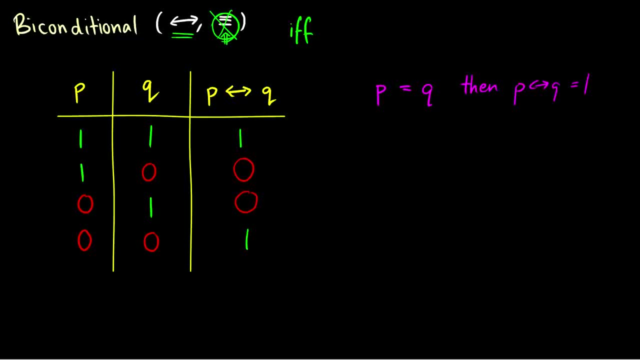 That's the biconditional. Finally, we have exclusive order, And exclusive order is really our idea of what or means in English. So this is the opposite of the biconditional. So if P is not equal to Q, then P exclusive or Q is equal to 1.. 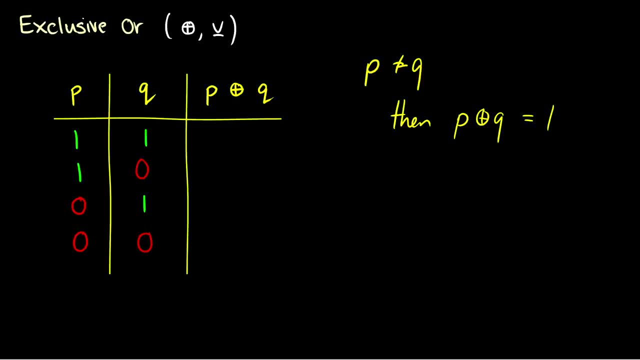 And typically we see it with the circle, with the line through. We might also see the disjunction with the little underline. Both are commonly used. I like the circle because it's very obvious that I'm talking about exclusive or And we also use the same symbol in set theory sometimes. 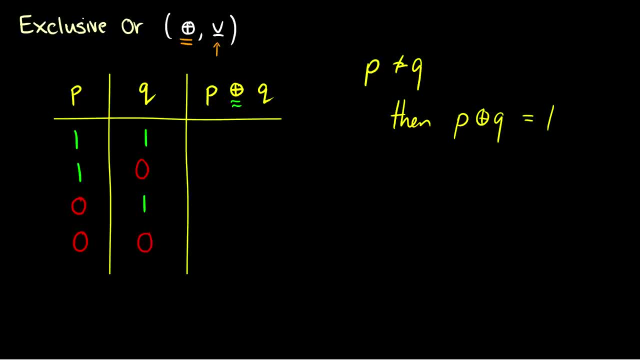 So it's just the opposite of the biconditional. So P true and Q true means that P exclusive or Q is false, And similarly, if they're both false, then that also outputs a false. But if the values are different, such as in rows 2 and 3, we get true. 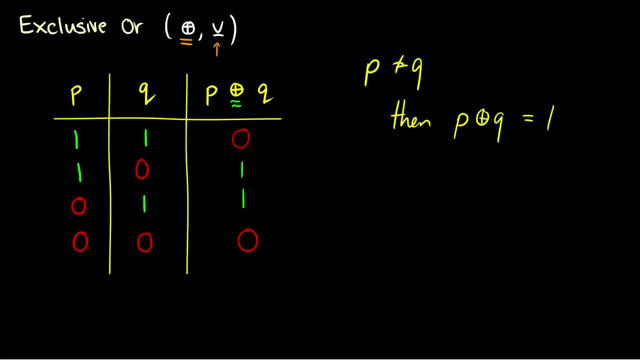 So those are truth tables, And in the next video we'll learn how to use these connectives and truth tables to prove that two statements are logically equivalent.